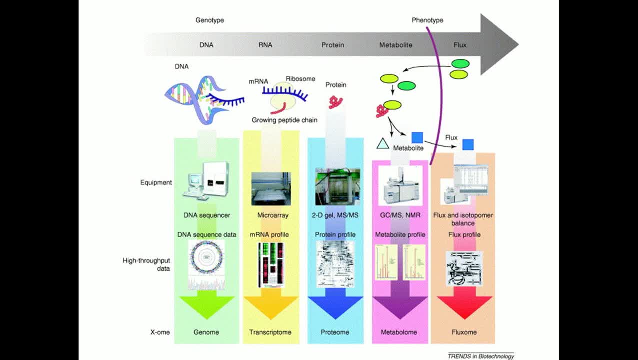 we have in our body, And then another thing is the phenotype, which we can observe from outside. that is a phenotype. So these are the two things: genotype, which is the inner side. phenotype, the outer side that we can see. So whatever thing is there inside our body, inside the genes, in the DNA, is actually controlling. 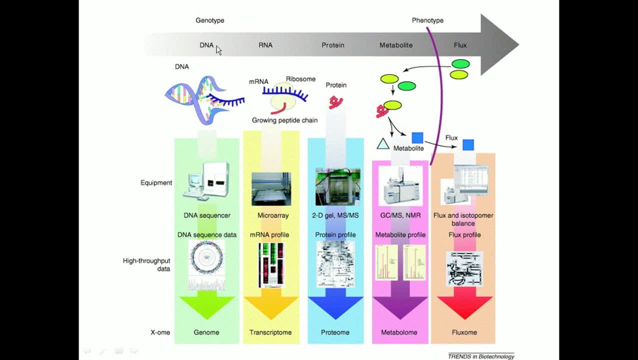 what is going to be our phenotype. So if we make a journey from genotype towards phenotype, what different molecules we encounter? For example, at the very beginning, genotype means the study of genes and the genetic makeup. That means the chromosome and inside that, 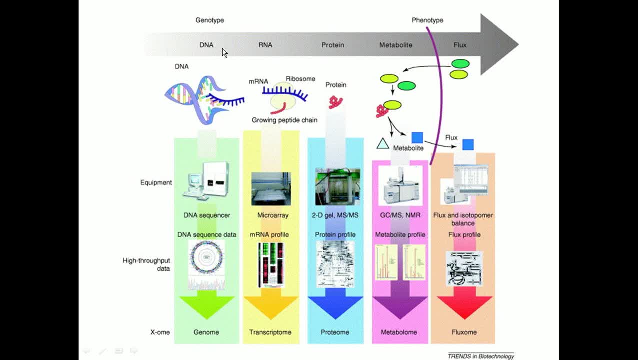 the DNA in the DNA, the gene. So that is belonging to the genotype And if you go slightly downstream of it, that means once the DNA is there and there are RNAs that are being produced from DNA Which are the messenger of the DNA sequences or the messenger of the DNA codes that are 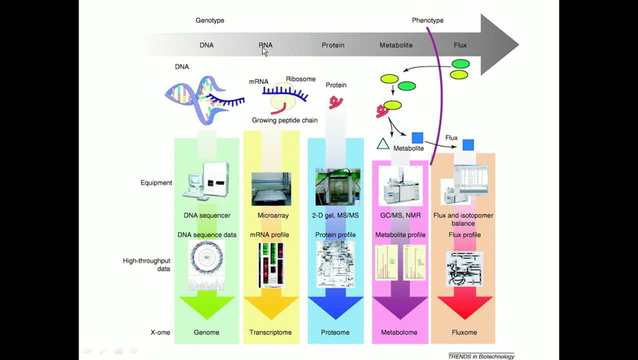 written in the DNA, So those RNA is there And the study of RNA and related to all the RNA molecules that are present in a cell or in a specific condition inside the system is called as transcriptomics, Because all the RNA that are present inside the cell at 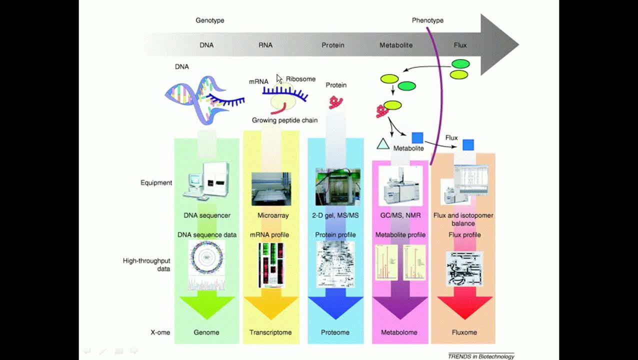 a particular time or in a particular system will be termed as transcriptome. So once you know that, those RNA will be translated into proteins. So now we have proteins, Protein structures, protein functions, So all the proteins that are present inside the cell at a particular consequence, at a particular time or- let's. 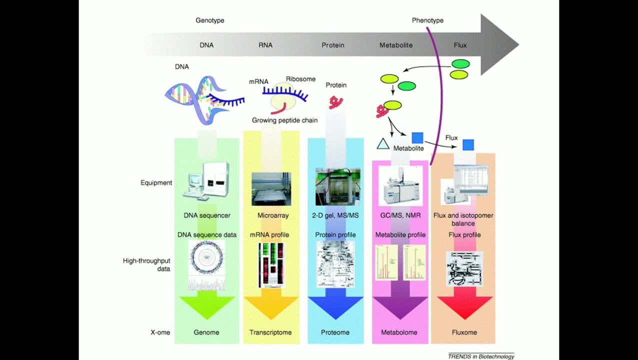 say in a particular system that is called as a proteome, The whole system of proteins that are present is called proteome And the study in which and the discipline of science and discipline of biology in which we understand the structure and function of all the proteins, 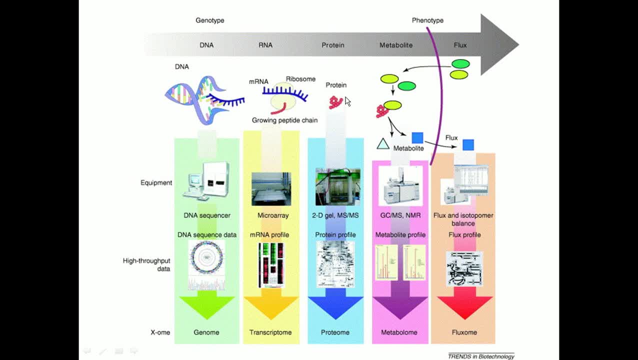 that are present inside the cell will be called as proteomics Right Now. after that, once you go from proteins to the metabolite level, let's say those proteins and they interact with each other- the protein-protein interaction and all those chemical reactions. 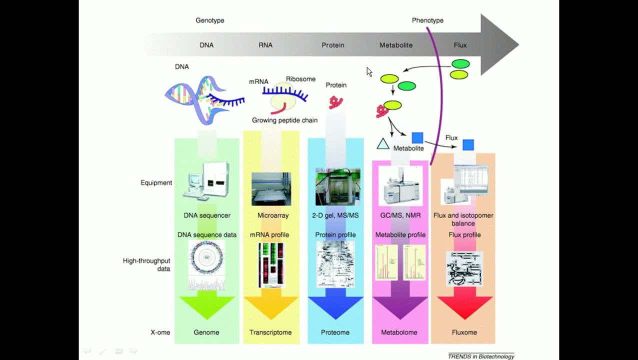 that are going on inside our body, like the glycolysis, like Krebs cycle, like many metabolic pathways, and they are related with each other And this whole metabolic system inside the cell will be called as metabolome of our cell And the study related to that will be called 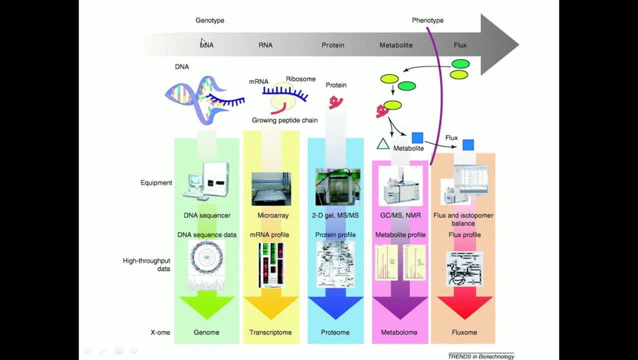 as metabolomics. So that's how you can see from DNA to our cell. that's how you can see from DNA to our cell, DNA to RNA, to DNA, to protein, to metabolite. we have genomics to transcriptomics, then proteomics, then metabolomics. So now let's move onto Now for each of this discipline. 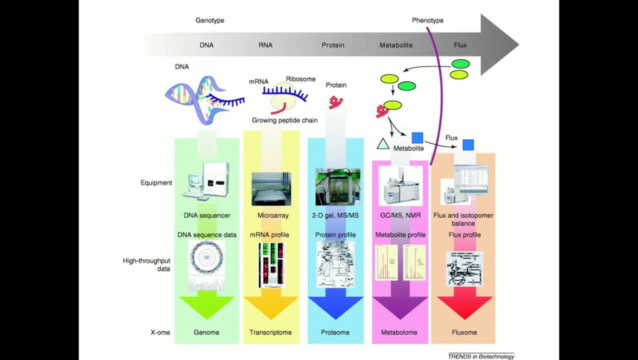 like transcriptomics, metabolomics, proteomics, genomics. we have different types of equipment. We require different types of equipment to actually analyze our results. For example, if you are looking for proteomics and understanding the protein structure, we need certain type. 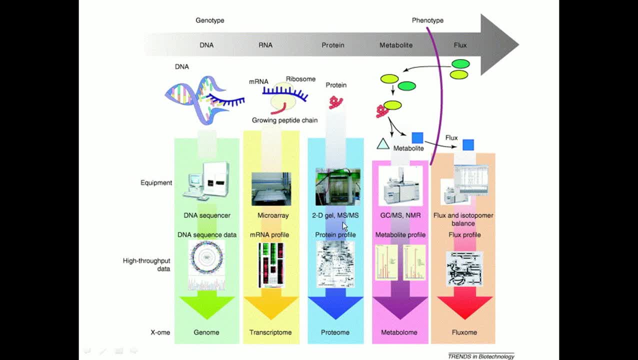 of setup- for example the mass spectrometry, two-dimensional gel electrophoresis, for example, process, other types of gel electrophoresis process- to know, so that those are the equipment that we require, and also we need to analyze some data to finally understand what is going on there, right? so? 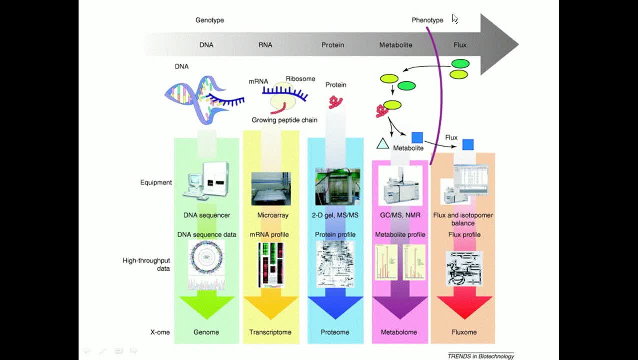 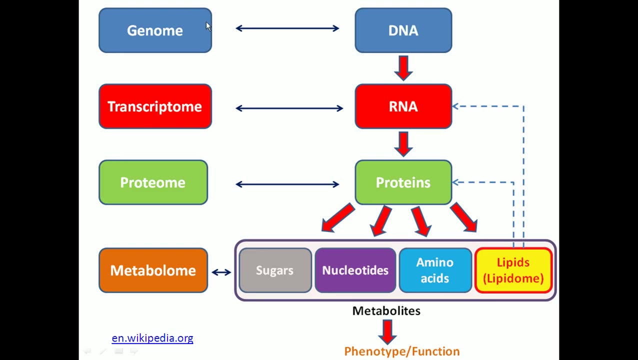 this is the actual link. we are going from genotype to phenotype. during that time, we are studying all these different phases like DNA, RNA, protein and metabolites, and we are using different equipments to do so. so now let's talk more about it in schematics. if you see, the DNA means genome here. 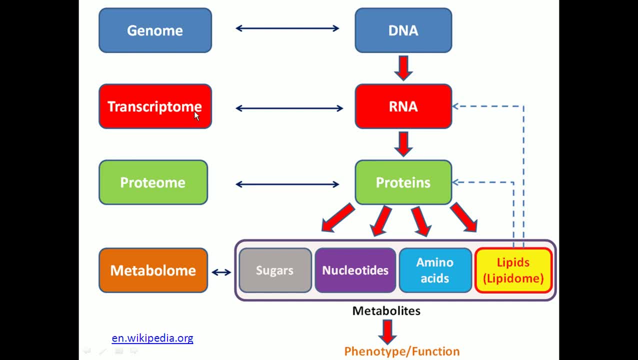 so genomics, RNA transcriptome deals with transcript to mix proteins, deal with prote suits, proteomics and, in the metabolome, inside the sugar, nucleotide, amino acidvocate ins, all the metabolites, all the macromolecules and how they interact with each other. and we are going from the genomics towards. 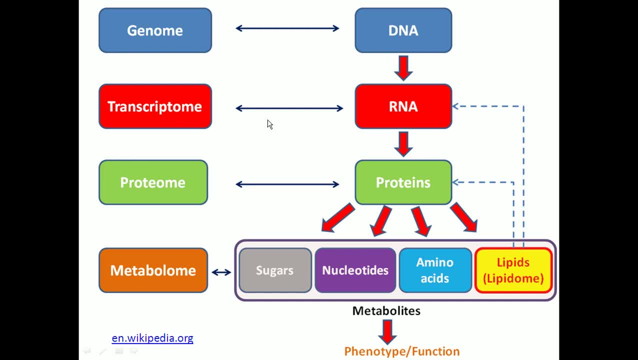 the phenotype, remember. so let's talk a little bit about each of the definition. what is Genomics actually? in simple words, genomic is a discipline in Genetics that applies the recombinant Dna technology of the DNA sequencing back system, so that this Archive can take you into the case which. 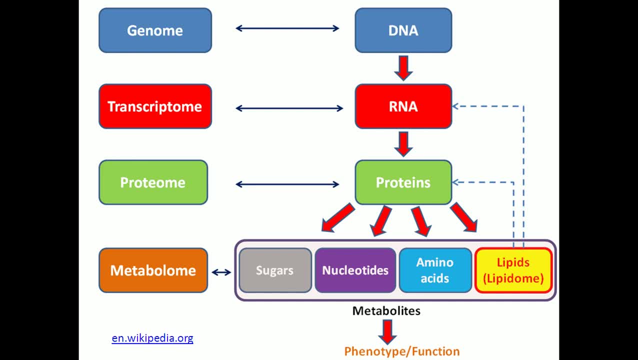 also diesemuch that applies the reconnaissance, Vietnam d' tournament, or the disease, sequencing, though you know, basis and when you wish you sm vastly genes, and now from the Miто, if you look at methods and as well as the bioinformatics, to sequence, assemble and analyze the function. 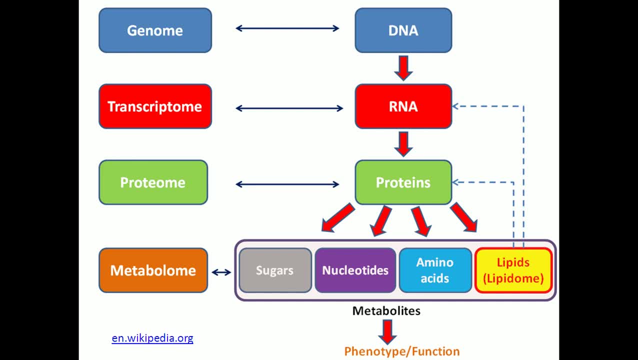 and structure of genomes. that means the complete set of DNA within a single cell or an organism, whatever right. so we actually understand the gene structure there. and the second one is the transcriptome. and what is transcriptomics? transcriptomics, actually transcriptomics, is a study of the transcriptome. now, what is transcriptome? the transcriptome here? this is that means. 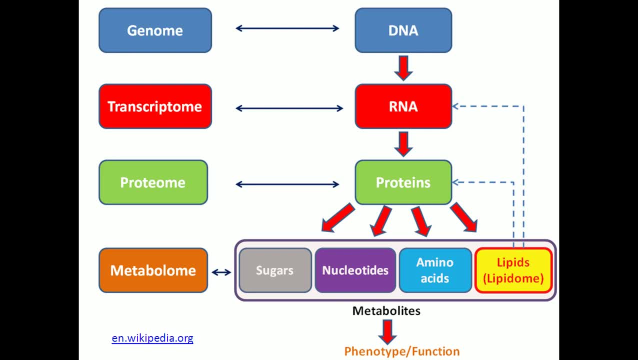 the complete set of RNA transcripts that are produced by the genome under specific circumstances or in a specific cell, and we use high throughput methods like high throughput sequencing and also microarray analysis, to ultimately know what is the transcriptome structure and how the function of transcriptome is going on in a particular cell: the proteomics. this is 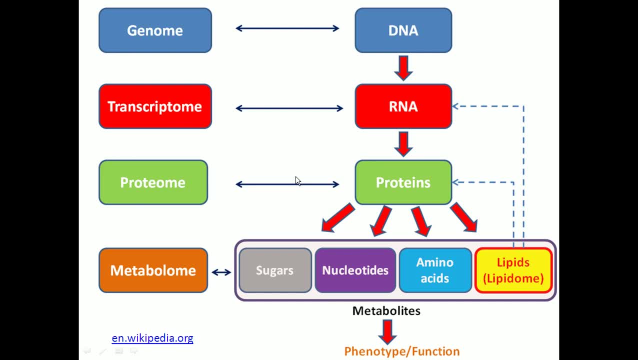 in a large scale study of proteins, particularly their structures and function of all those proteins, their motives, that domains how they function. then the metabolomics: at the end it's a scientific, again against the scientific discipline, to study the chemical process involving metabolites inside the cell, specifically metabolomics. 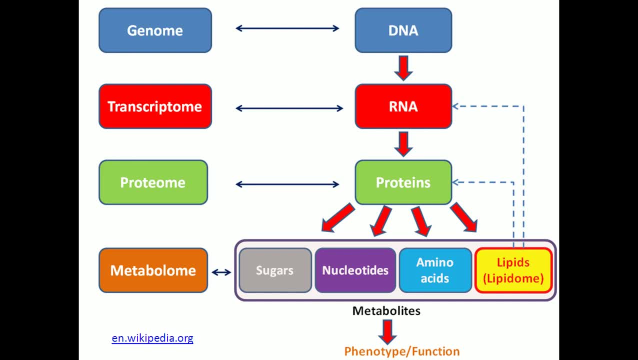 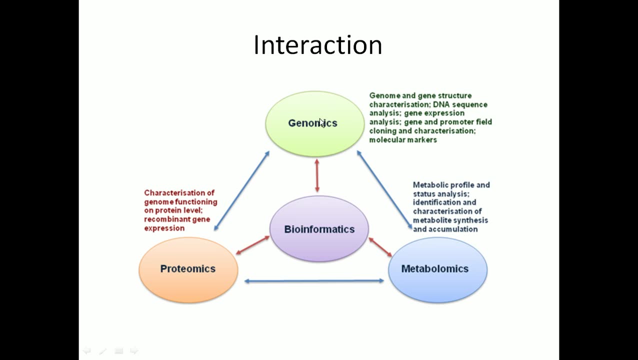 means, you know, systemic study of unique chemical fingerprints that specific cellular process leave behind during different metabolic reactions. right, so now these are the interactions between all them, all of them, like the genomics standing there with DNA and RNA structure, the genome structure. the characterization of the DNA, like the DNA sequence. analysis of the DNA, like the. 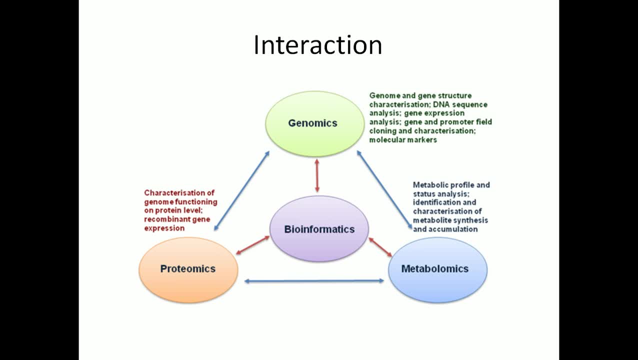 gene expression and cloning and characterization and molecular markers, all of these things and related the study. all of these things will be related with the genomics there, right, everything that along this part inside genomics. then we have the fruit, then we have the proteomic. said that the 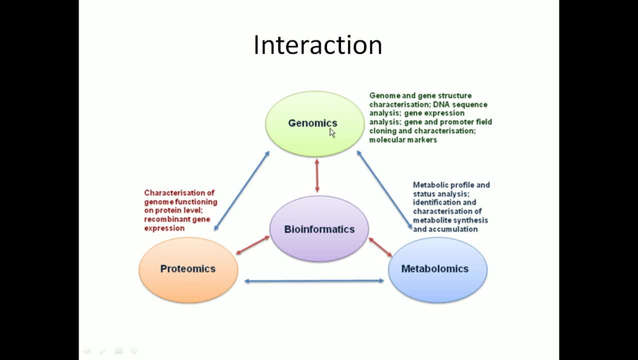 characterization of the genome function and the protein level. expression of and the analysis of those genome expression in the protein level will be proteomics and the metabolomics is the metabolic profile, like the status analysis of a metabolic pathway, the metabolic synthesis and accumulation. everything under this will be metabolomics and you know all of this: like genomics, proteomics, metabolomics. 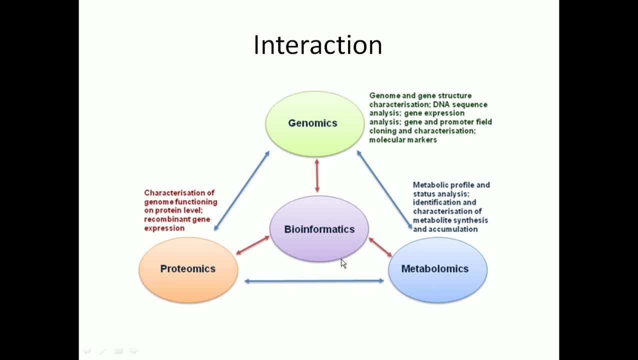 and also transcriptomics, which is not shown here. they are ultimately relying on bioinformatic analysis, because the bioinformatics is a tool which can connect all of these things together to give you a solid understanding of what's going on inside the cell. if you look at the connection, 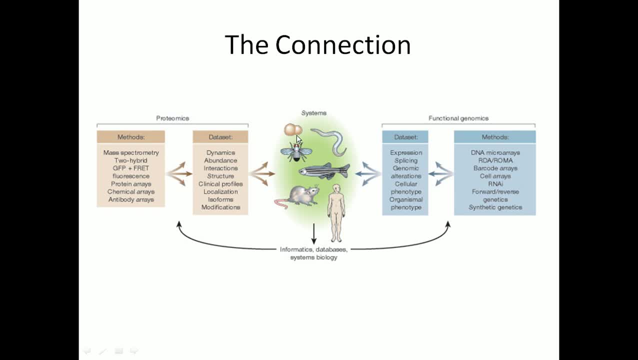 here you can see this is a system. what kind of system? it is anything like like, let's say, the East. it's a very simple eukaryote or a drosophila or C elegans or zebrafish or the mouse or human. 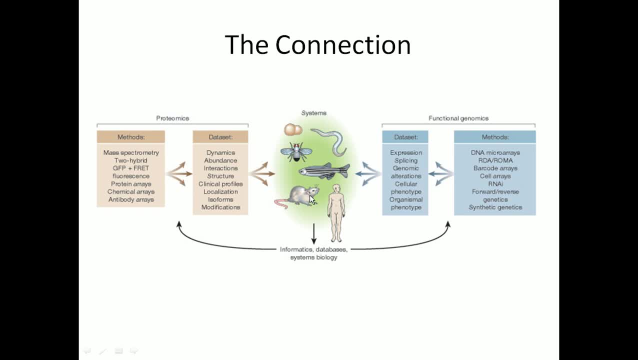 whatever it is, they are the model organisms that are present, whatever organism that there is, whatever organism is present. we have all this idea, like, like you know, in proteomics, why we want to see the isoform of the proteins, the dynamics of the protein, the interaction between proteins, the structure and function of the 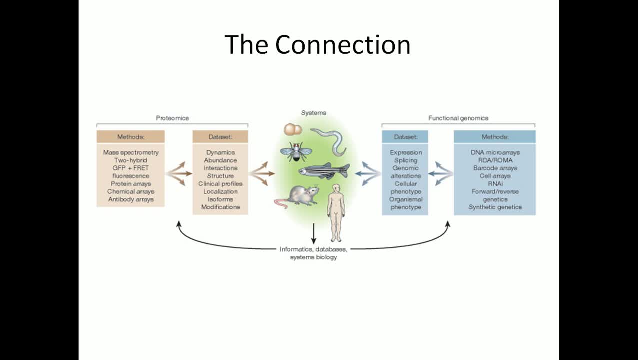 protein, modifications of the proteins. and to understand all these things we need to rely on certain methods and, obviously, certain machineries. the methods here are: we use for the proteomics study our mass spectrometry East to hybrid system to find out the protein protein interaction. then 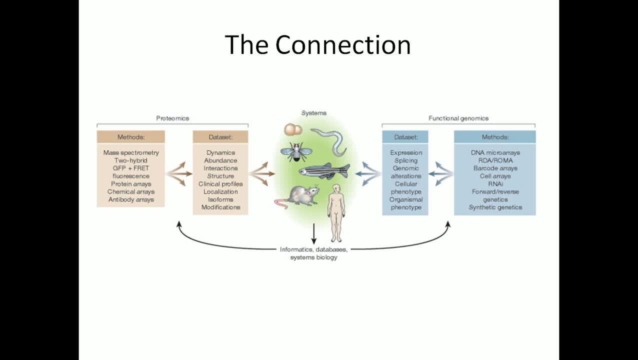 the GFP fret: the green fluorescent protein identification, the confocal microscopy to see the fluorescence analysis, the protein arrays, then chemical arrays and the antibody arrays to identify all of these things. right, so these are the different methods that we rely on to study proteomics. on the other hand, if 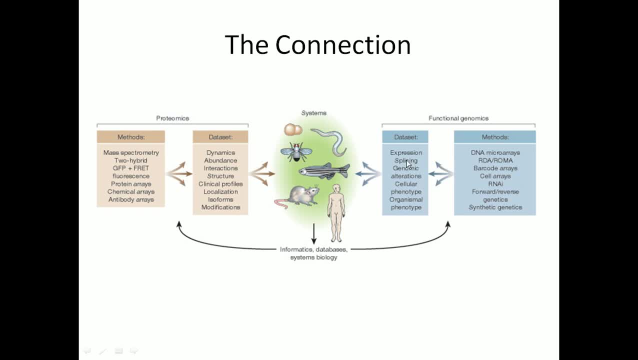 we look at the genomics part, the genomics- we deal with the expression of a gene, size, splicing of the gene and the genomic alterations, cellular phenotype and and all this how, how these genomes are actually relating with the phenotypic expressions. so all these things related to genomics, and actually the genomics, can be divided into: 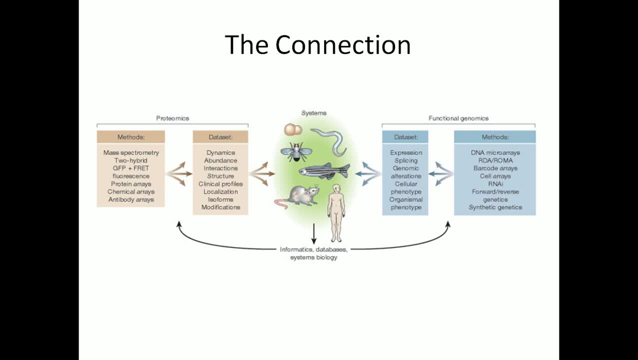 two part: the structural genomics and the functional genomics. the structural genomics is to deal with the structure of the gene, whether there is intron or exon and how they function, how the splicing is going on, why splicing occurred and what are the different variations of the same gene can 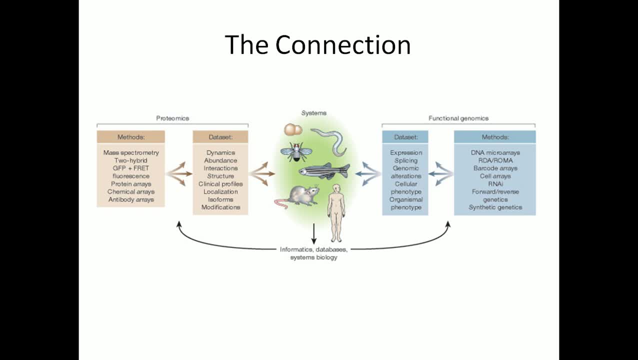 be possible. on the other hand, the functional genomics look at the expression of these genes and all the genomic analysis systems. and also we need some methods, other methods to know, some other techniques to understand, and those techniques are DNA microarray system, DNA barcode analysis system, the barcode. 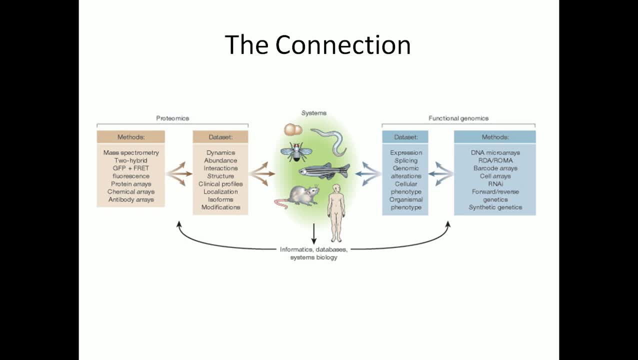 array is, the cellular arrays are an interference machinery: forward and reverse genetic, synthetic, synthetic genetics and all these different kind of methods and also equal different techniques and different machines to. I actually get that data microarray analysis machine and all the things right. so these are that this is the connection of a particular system with. 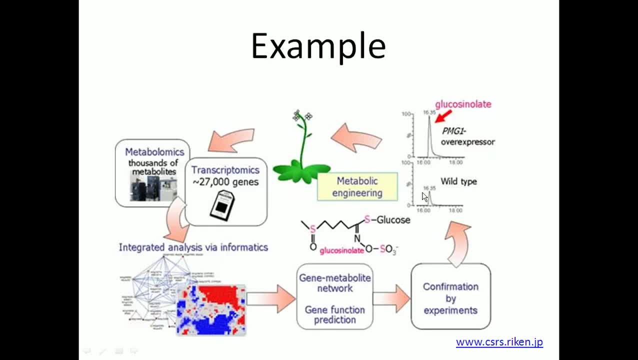 all this: genomics, proteomics or transcriptomics, whatever we are talking, and this is an example of all this process and how this process actually works. if you start with this, let's say this is a plant, Arabidopsis thaliana, for example, we begin with this particular plant. now we need to look for are the 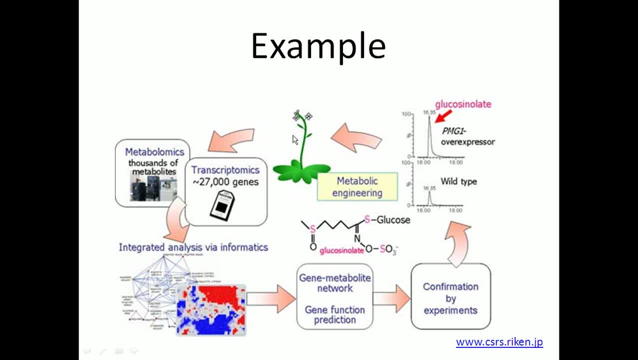 whatever proteins or whatever whatever RNA, the total content of RNA that is present in this particular plant. right? so actually, let's say we want to understand what is the protein that is there which helps this flower at this, this plant, to provide the such a beautiful plant, which helps this flower at this, this plant, to provide the such a beautiful. 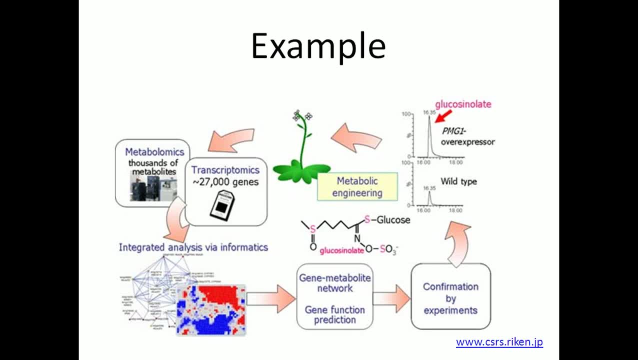 colorful flower. so to understand that, we need to know what are the mRNAs that are coding for those proteins. so we need to look for the transcriptomics- and there are 20,000 approximate genes are there and we need to find out what are the different RNAs there and how they are interacting with each other and we 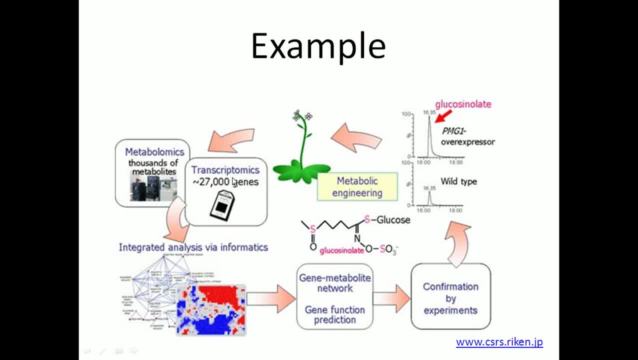 use transcriptomics analysis to find that out using DNA microarray. so once you understand that we, we add it with the bioinformatics, we integrate with bioinformatics analysis to get a result. so once we get the result, what we now need to know, we need to know we need to go for the DNA. I mean gene function prediction. 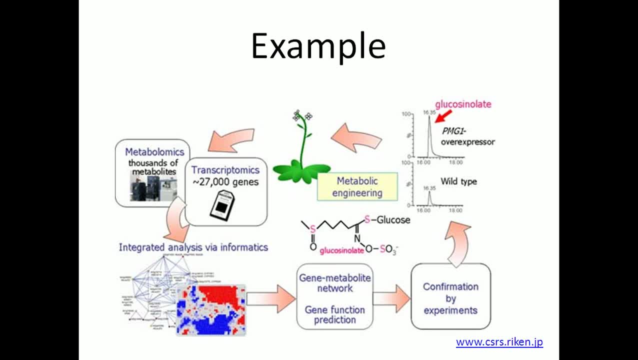 we can predict the gene function. what can the gene be? I mean what? what is the function of the gene? by simply integrate this results of transcriptomics with bioinformatics, and once we know that this gene might be related with some kind of- what expression analysis protein like PMG1. so let's predict that and find that. 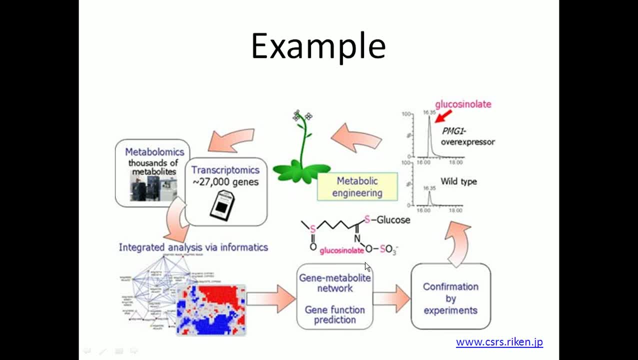 out. so we need to confirm that process and we then go for the, the identification of the protein level, and we need to check for whether that protein is presentable or not. or not we extract that protein, find the proteomic analysis using mass spectrometry and uh 2d gel. 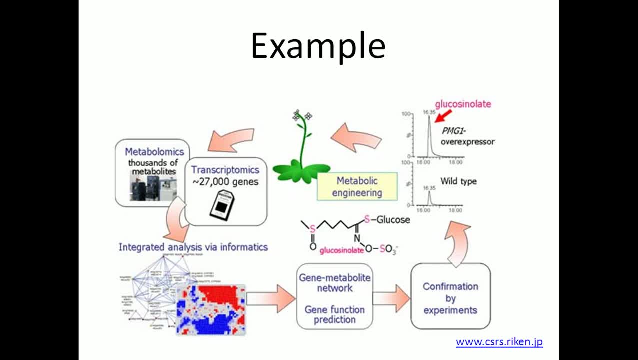 electrophoresis and other processes to find out that protein. now, if you find that protein out, and we can also find that proteins- importance during the process inside this, inside this plant, uh, to find out whether the the length of the plant or the power flower, flower color of the plant.